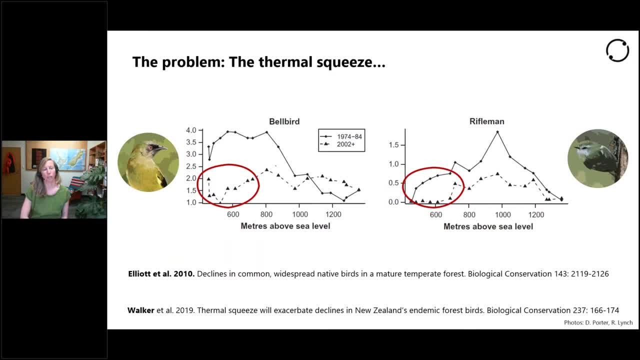 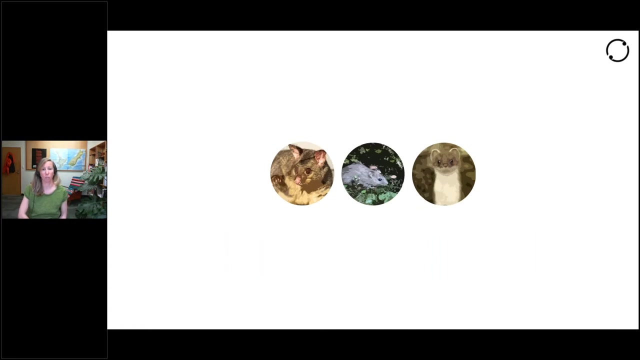 native forest birds decrease, particularly in more warm, floristically diverse forests, and this problem is of course of huge concern but also may pinpoint towards where we could make the greatest difference for population restoration. As John touched on yesterday, the primary limiting factor of native forest birds are introduced mammals. I've put up here possums, rats and 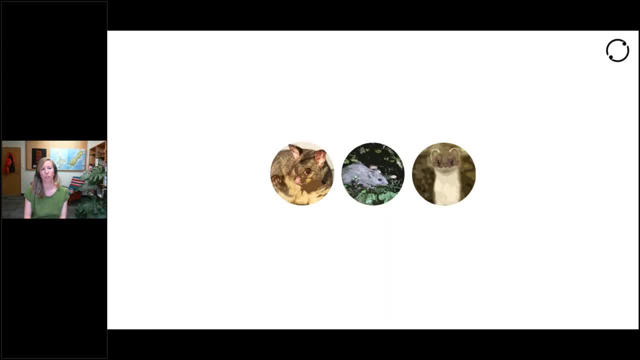 stoats, but of course these are not the only ones that cause havoc in our forests, As we again heard yesterday quite extensively. the resources and time and space drive the population abundance of these introduced mammals and they of course prey on native bird populations but also consume food. 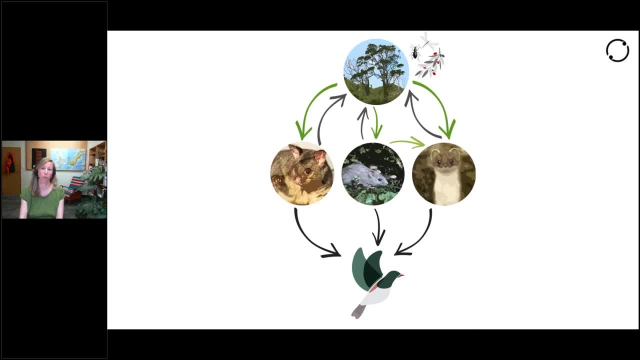 resources that would otherwise be available for native birds. So they're predators and food diverters When, under high abundance of introduced mammals, food resources are likely to have only a minimal effect on vital rates of native forest birds. So by vital rates I mean fecundity, juvenile survival and adult survival. 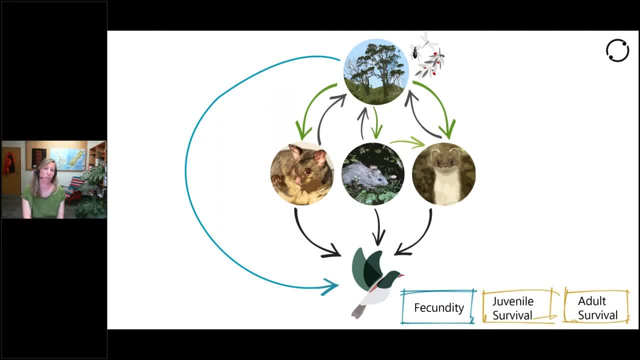 And that is because most breeding attempts are just terminated by predation, and so it doesn't really matter how many attempts are made or how big a clutch is, if the end result is that none of those eggs ever hatch. And similarly, juvenile and adult survival, depending on the species, can be significantly reduced by high. 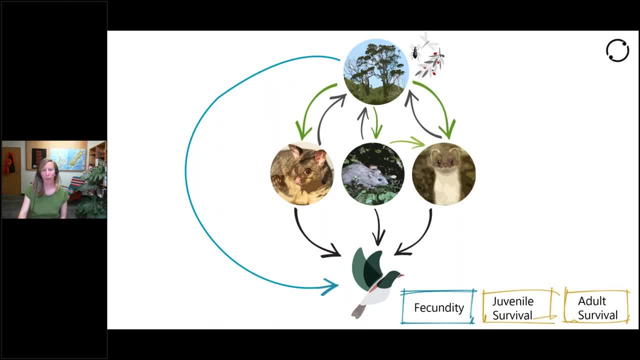 abundance of introduced mammals. However, if those introduced mammals are suppressed, food resources may play a much bigger role in driving fecundity, juvenile or adult survival. Currently in New Zealand there's little. this is actually a bit of a knowledge gap that we 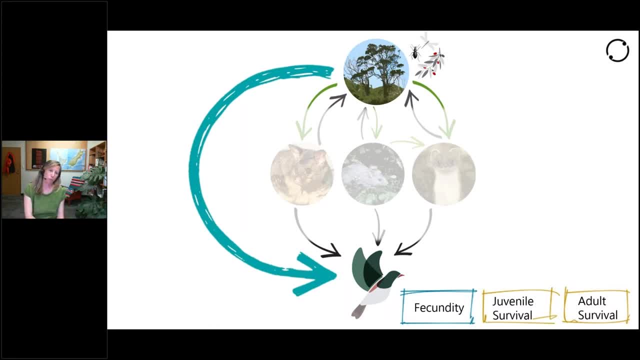 don't understand that well in which way food resources influence fecundity or survival, And I wanted to address this knowledge gap using a large scale field study and focusing particularly on the smaller rat sensitive species. So these are mostly insectivorous passerines that are sort of 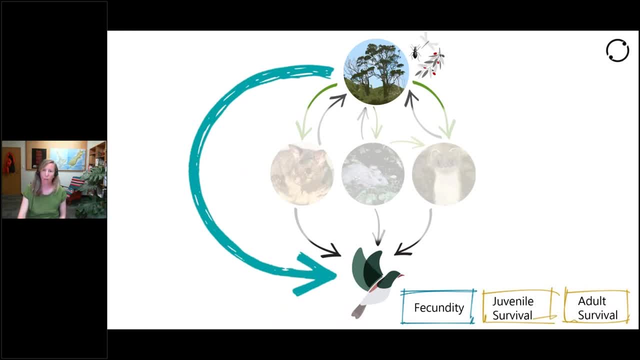 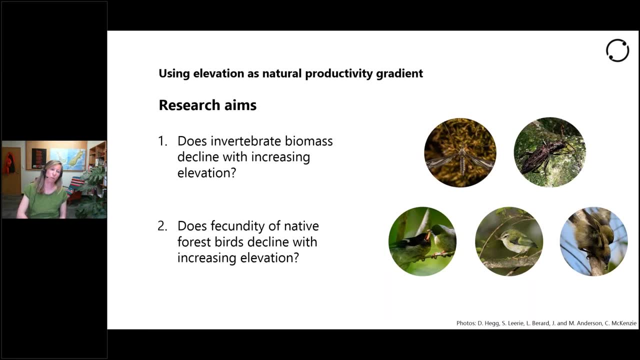 smaller than about 35 grams. I wanted to use elevation as a natural productivity gradient and first answer the question of if actually along that elevational gradient, this presents a gradient also in food resources as well. And for example, do vertebrates have more land? Hahnicki, we think that this is 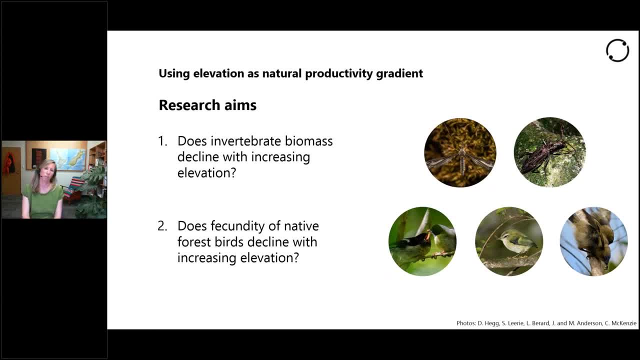 actually equal to maybe nine tick or at least one thousand species that have been harboured by formation of a second and third gen invertebrate. So you know first off how explode or balance of these species really gives utions in general, and also how can a population change and gently change. 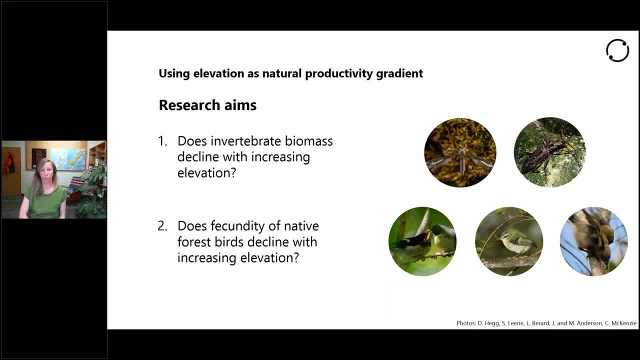 from you know, looming vertebrate being what we normally would call an textile sixteen age range is significantly different from what's would be in between. So those small body species, seeing that the number of insemination mutations increase, inalf the species being pred钱, hugo cooling. 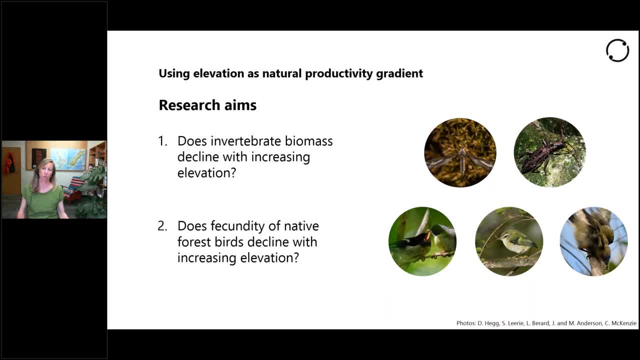 with a really long-lived species like albatross, survival kicks in and driving population dynamics quite a lot more, but with smaller species that have a shorter lifespan, fecundity can have a huge influence on population dynamics, and so I focus much more on fecundity. I chose three species. 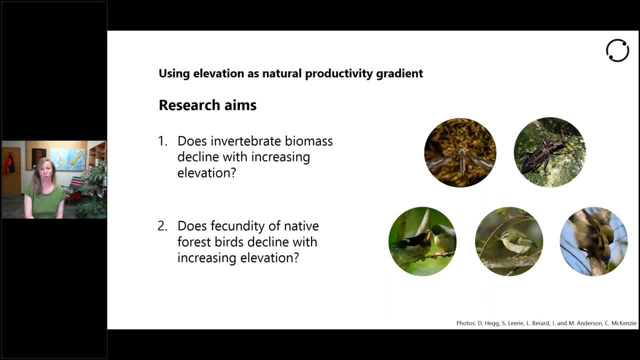 as case studies: Miro Miro, Tomtit, Titiponamu Rifleman and Korimako Bellbird. All of these species have significantly reduced abundance and distribution since human colonisation, but are also still actually able to coexist in forests with introduced mammals around, and therefore they 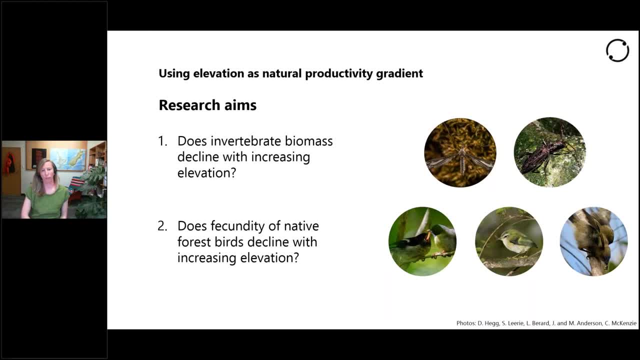 also have the potential to hugely benefit if we can get the pest control right and be able to restore populations. The other aspect that I took into account: that those three species have slightly different life history traits and vulnerabilities. so, for example, their nesting habits- from being whole nesters or open-cap nesters, differ and, for example, their size is different. 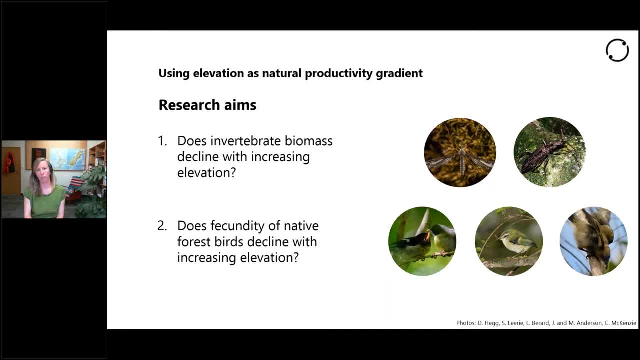 And so I wanted to know if actually the responses are the same across those three species or if they differ between the species. Unfortunately, despite huge field effort in trying to find Bellbird nests, we were only able to track one female to a nest, and therefore I'm not going to talk much more about Korimako for the 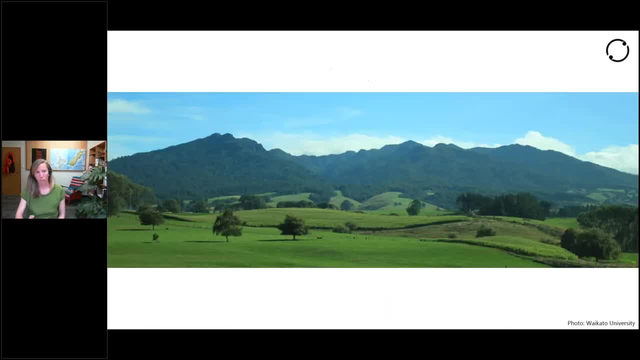 remainder of the talk. This is the place where that we used as a field study, that's Mount Porongia, near Hamilton in the Waikato. It provides an amazing elevation gradient but, as you can see, the lowland forest is cleared, so we try to get the maximum. 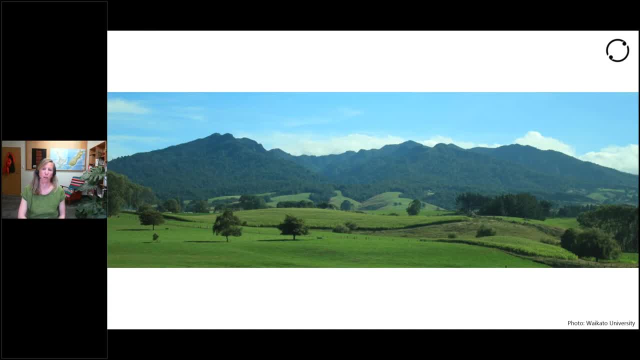 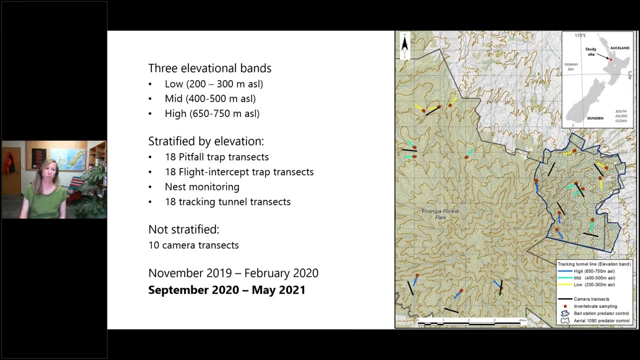 elevation gradient that we could, but we weren't able to go right down to near on sea level just because there's no, no forest left, unfortunately. We set up the study in three elevational bands, so at low, between 200 and 300 meters, then a. 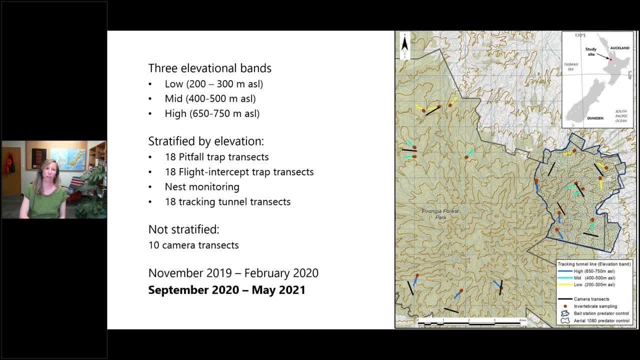 mid elevation 400 to 500 meters, and then a high 650 to 750 meters. Across these elevational bands we sampled invertebrates and pitfall and flight intercept traps. These were run throughout three seasons, so spring, summer and autumn, and always left open for about a month. 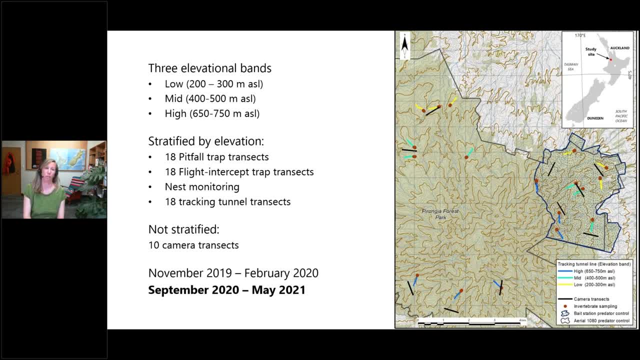 And also we monitored rodents using tracking tunnels and then stoats and possums using camera transects. Those camera transects we weren't able to stratify into elevational bands, because then they wouldn't be independent anymore, so they were just randomly allocated throughout the site. Our initial field season was cut short. 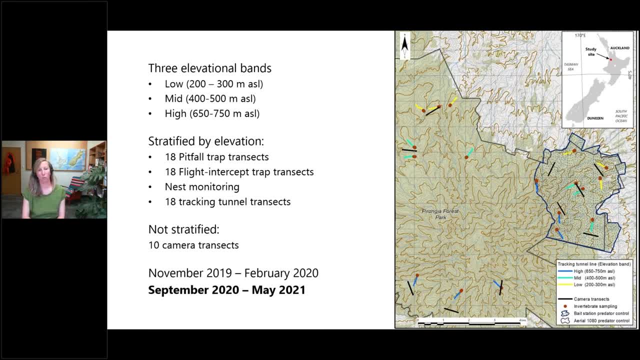 or actually rather started a bit later rather than cut short due to a delay in getting our wildlife permits, And initially we had set up one site that received predator control in the form of a bait station network that is serviced by the Porongia Restoration Society. 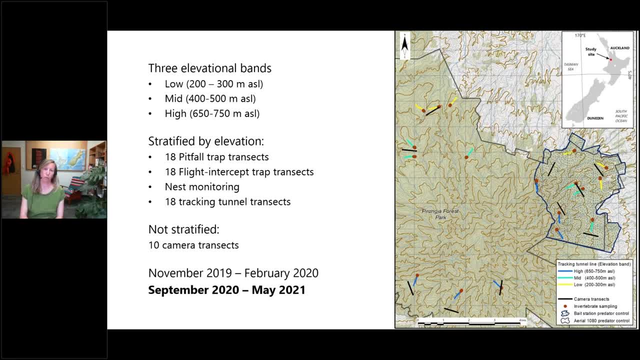 And a non-treatment site, which was the remainder of the Porongia Forest Park. The second season the remainder of Porongia Forest Park received a 1080 treatment. so in the second season the entire study site was under effective pest control. Due to the small sample size from. 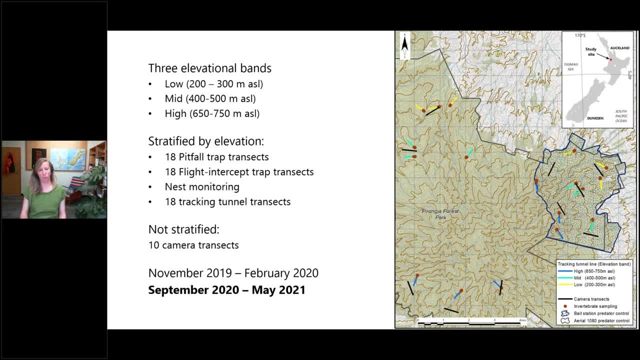 the first season. I'm only actually going to present results from the second season and present all results together. So I'm just going to show you the data, because our data show that pest mammals were effectively reduced across the entire study site and all elevational bands. 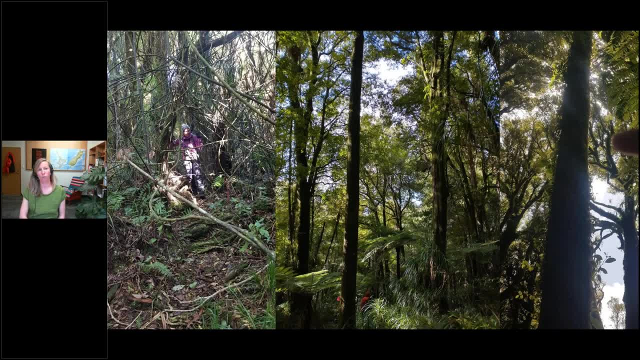 First let me take you into the field. So a combined 4000 hours of field time made us experts at navigating supplejack patches and looking up, up, up and up. So right at the bottom of your screen you can see a person doing a. 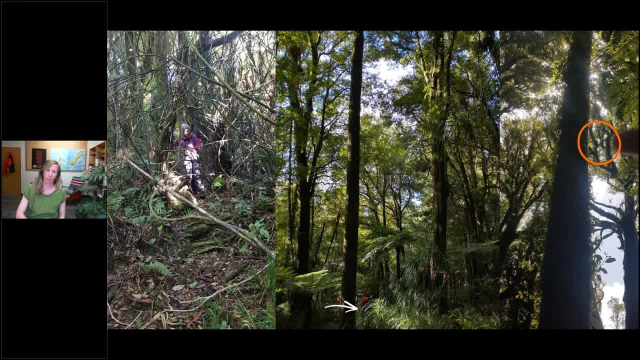 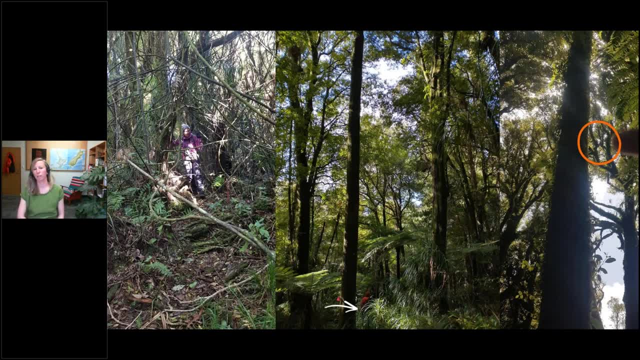 sometimes over 15 meters and you could just make out a changeover in incubation duties between riflemen or if it was tomtit the male calling off the female for feed. But we got just shy of 100 nests in that second season and it definitely was those exciting days. 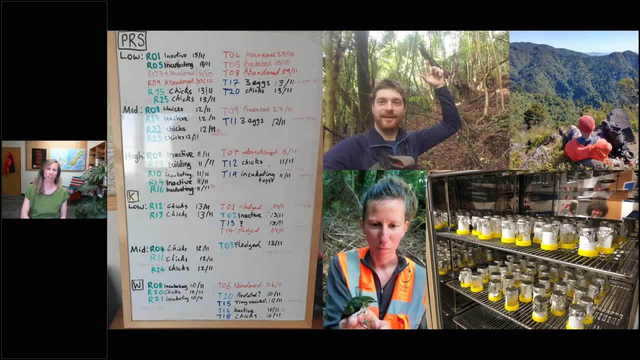 when you do actually find that nest or get to have your lunch in the sun with a beautiful view and also get to finally sort through all of those invertebrates that were collected during all those times and see them all nicely sorted into the different size classes and orders. 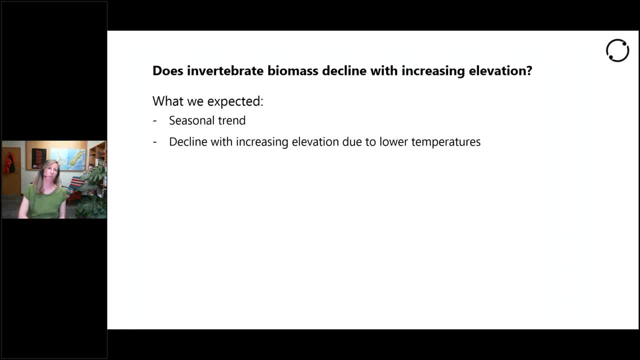 Back to my questions. So, first of all, does invertebrate biomass decline with increasing elevation? What we expected was that we would see a seasonal trend, so a higher abundance of invertebrate biomass in summer compared to spring or autumn, and a decline. 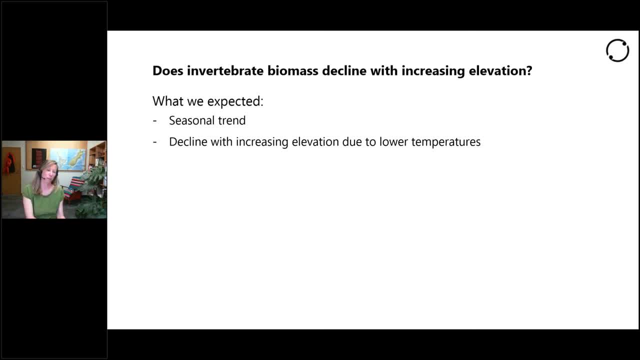 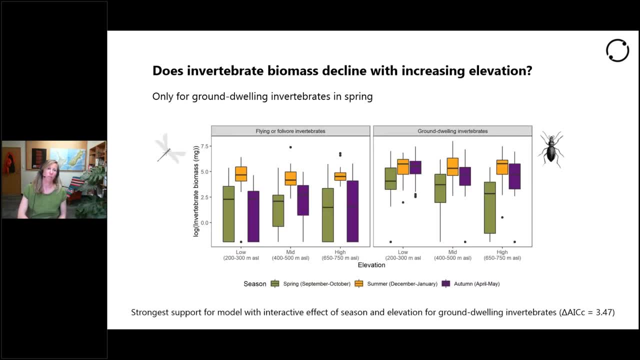 overall between elevational bands, so higher abundance at low elevation and lower invertebrate biomass at high elevation. What we found, though, was that for flying invertebrates we only found a seasonal pattern in biomass, so there was no elevational trend at all, And for ground trailing, 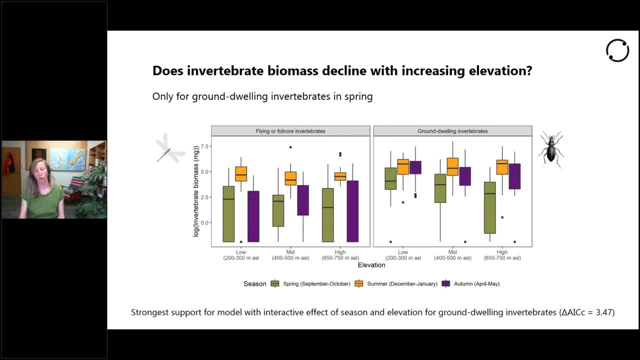 invertebrates. there was an trend, but only so in springtime. so you can see in green that is this: the spring samples and biomass actually decreases as you go up in elevation. so we have the strongest support for model with an interactive effect for season elevation and only for the ground dwelling invertebrates, but only a seasonal effect for the flying invertebrates. 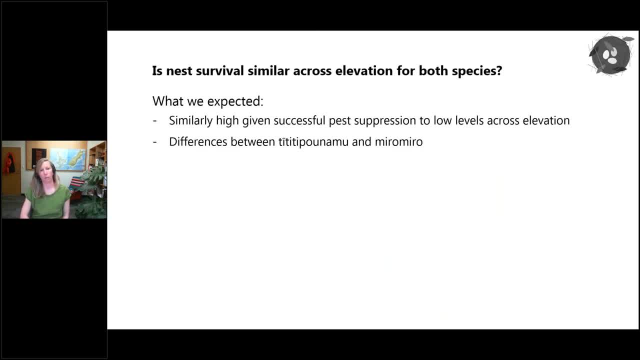 and so how did that look like for nest survival, and was it the same for both species? so we expected, given that there was a strong suppression of the key pests to low levels across elevation, that actually nest survival would be high and actually would be high across all elevation bands, and that there would be species specific. 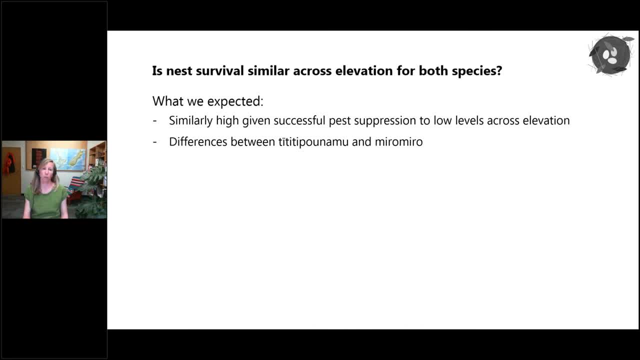 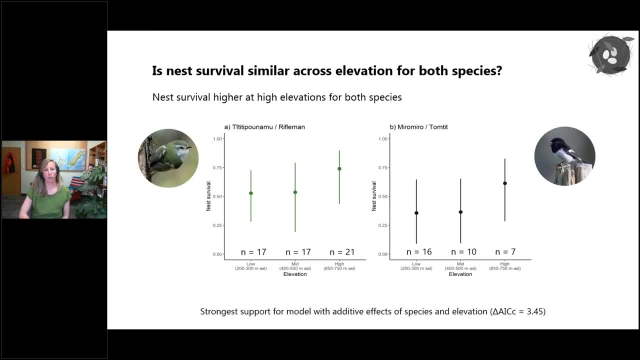 differences between titiponamoon and miromiro- potentially given that they've got slightly different nesting habits- and what we found was that the trend was the same actually for both species, which is quite cool, but also that nest survival was actually higher at high elevation. 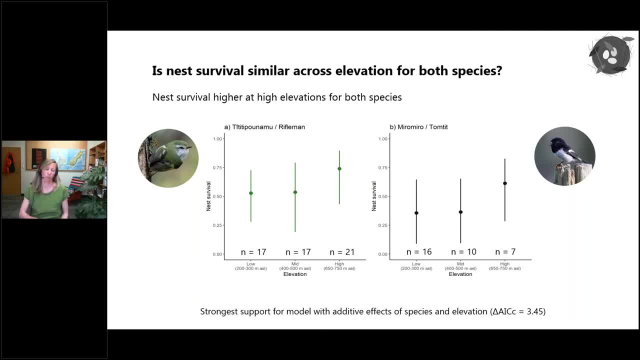 for each species compared to the lower elevation, so we had the strongest support for model with additive effects of species in elevation. as you can see, though, effect sizes are small and confidence intervals overlapping, so it's the suggestion of a trend, really. and how did this play out in the number of fledglings produced per successful nest? 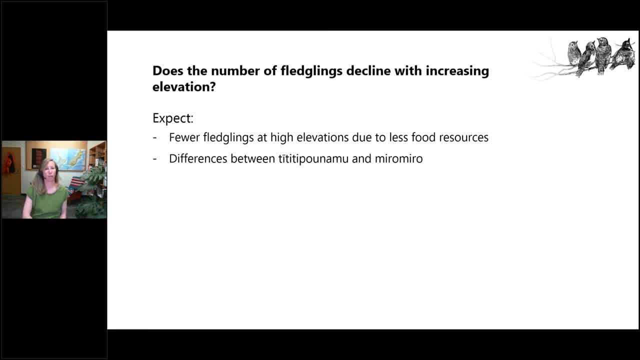 so we expected that there would be fewer fledglings at high elevation due to less food resources available to birds and, again, given the different clutch sizes, that there may be differences between the two species- titiponamoon and miromiro- and what we found was that, again, we had the strong support for model with an additive effect. 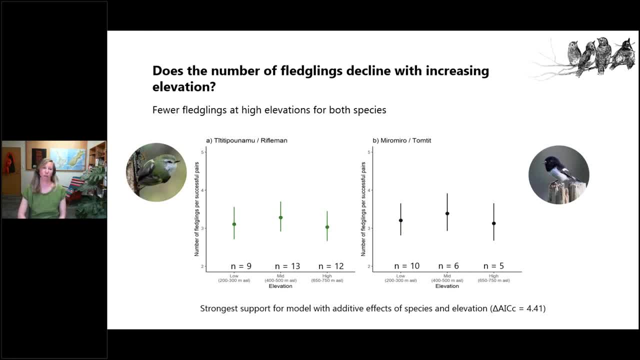 of species and elevation. so for both species the trend was the same, there was no interaction between species and elevation and that there was slightly fewer fledglings produced at high elevations compared to the other elevation bands. but again the effect size was fairly small and 95% confidence. 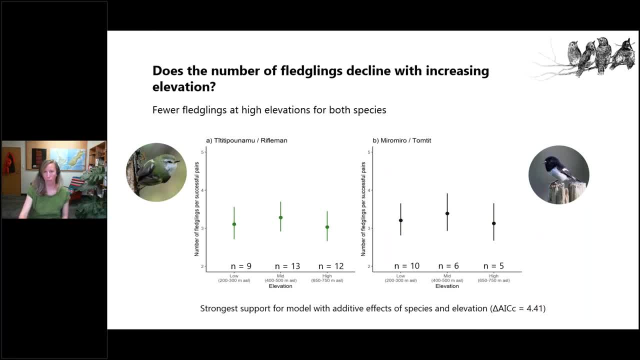 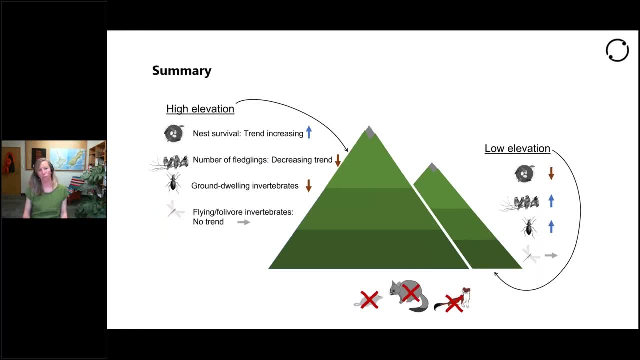 that we had between species and emission examples, and result of that was that stagiri fears that the agreement must be usually prepared so that we can consider the ervation, fishes and operation of ortu high elevation and fewer ground-twelling invertebrates available in spring, which is when primarily 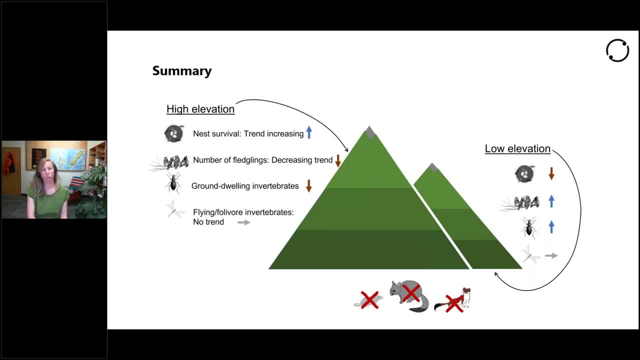 most of the nesting activity happens. There was no trend at all for the flying or foley wall invertebrates and we think that rain might be much more of a factor than simply just temperature, and rain would more evenly affect all elevation bands. The other point: 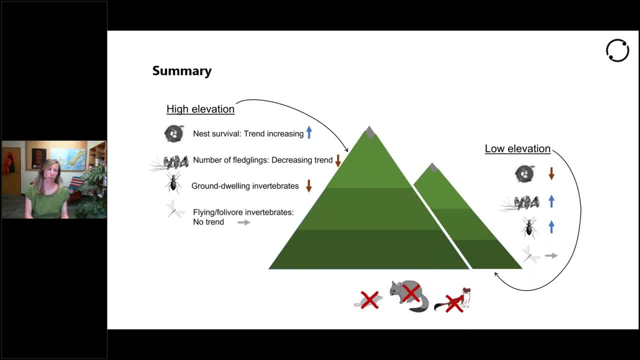 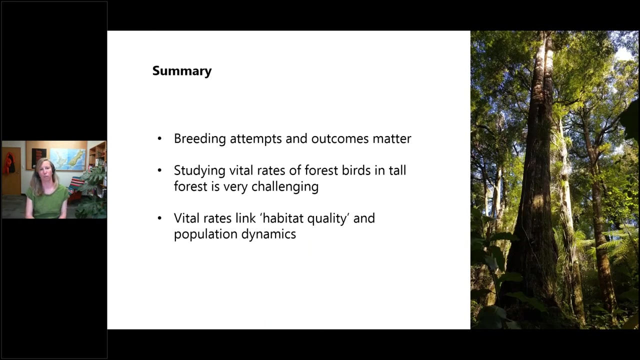 is that because our sampling window was a month, at a time that flying invertebrates may be, either by themselves or through wind, more easy to actually get up and down the mountain, and so any differences might be diminished through that longer sampling window. And again, to briefly sum up, so it's the breeding attempts that matter, which are primarily. 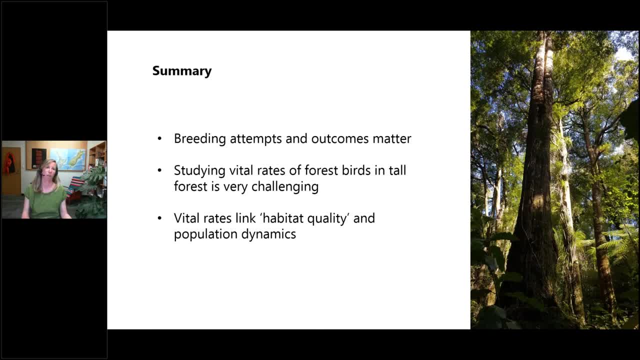 more food-driven as well as the outcomes. and so we have the first suggestion that actually there could be an elevational trend in nesting or in fecundity, nest survival and fledglings produced. but the study of vital rates of forest births, particularly in those tall 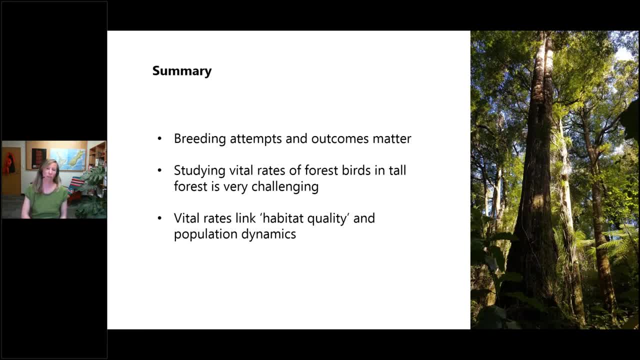 complex forests is really challenging and, yeah, really challenging. It requires quite a fit field team and loads and loads of time. However, on the whole, it really. those vital rates allow to actually link habitat quality and like what drives. 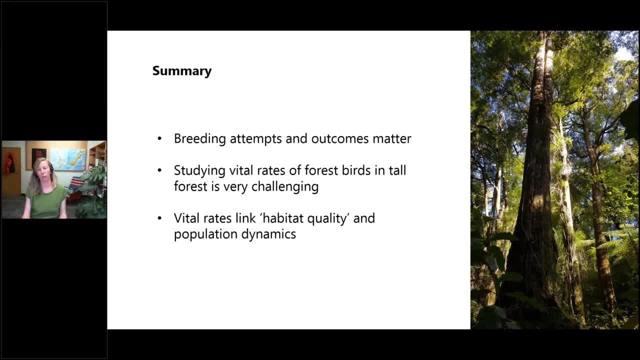 those population dynamics and you can actually understand much more of what is, yeah, good habitat versus bad habitat. And, as an exciting next step, there's a master student that will use, Yeah, an experimental approach in supplementary feeding, using an ecosanctuary site and a non-fenced 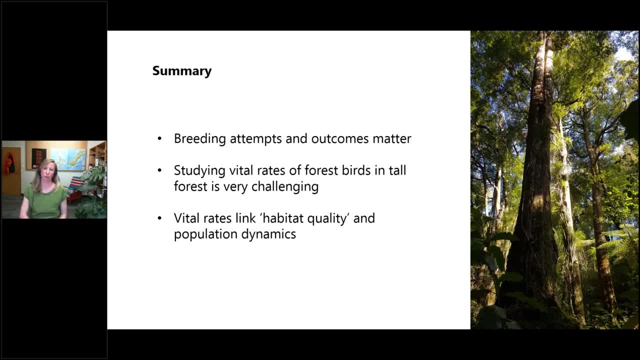 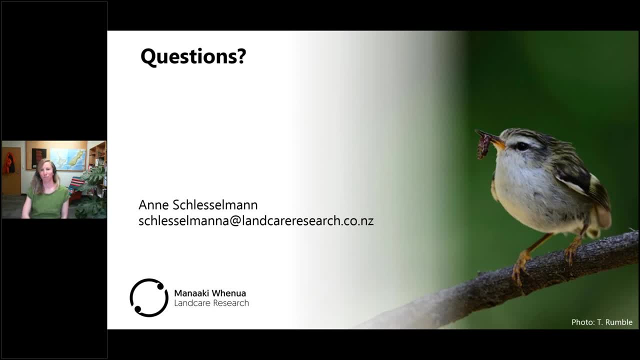 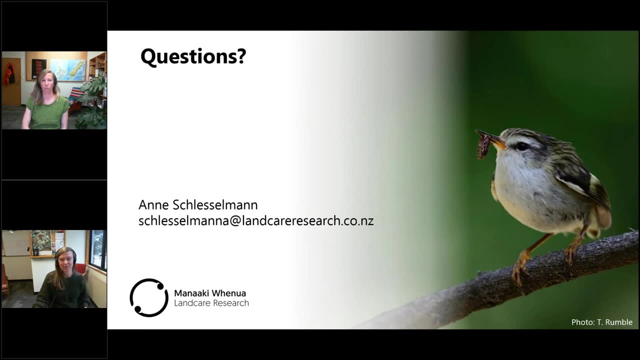 site to tease out even more how predation and food interacts. Are there any questions? Thank you so much, Anne. That was a great talk. You've had one question already, which was: did you measure temperature differences? Did you measure temperature differences at your sampling sites? 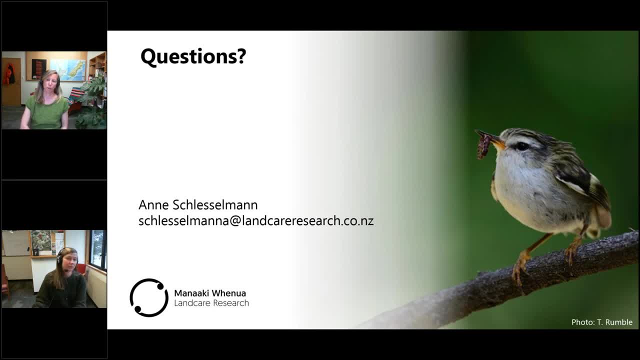 Yes, Yeah, we used little eye buttons at the same places where our rat tracking and the invertebrate sampling took place, And again we can see that nice pattern of that. high elevations never well, are always colder than the lower elevation sites, but there. 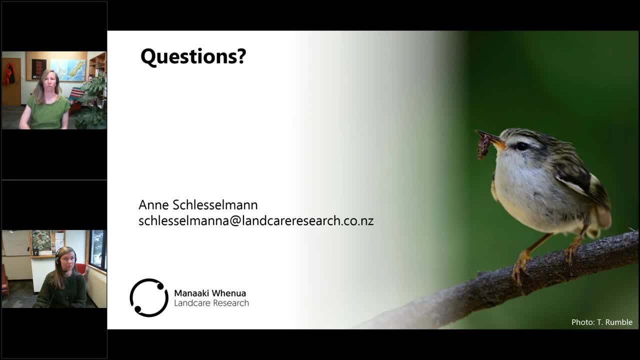 was only about four degrees difference between our sampling sites. So yeah, that's a good thing, Yeah, And actually a much greater seasonal difference between kind of from spring all the way through to summer and then back to autumn. I've got a question: How did you know whether the invertebrates you were sampling? how did? 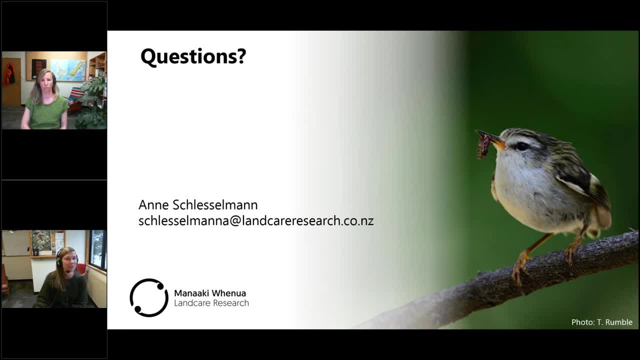 you know they were important to riflemen and tomtits and their diet. We- Well, actually I should say James, Yeah, Yeah, Yeah. So I think the things that we did- the technician and Scotch as well as Stephen Ford- were amazing. 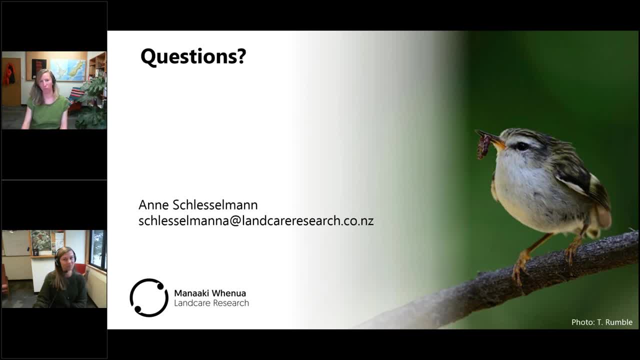 at actually sorting through all of the invertebrate samples and sorting them into different size classes, so that we could actually look at what would be, roughly, what we would consider actually bird food versus bigger items that would still be eaten by opossums or rats. 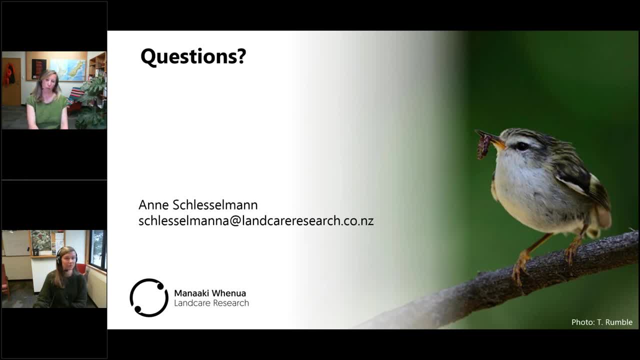 and then also identified them to order- Yeah, those orders. so we knew which orders were sampled and could go back to diet studies from back in the 80s and look at- actually also later by other people and where they documented what miromiro and teteponemur fed on and that 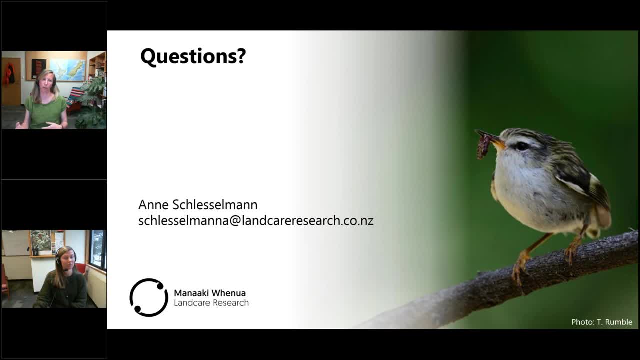 actually matched really well, although of course it's mostly a general measure of available invertebrates that we did, but they were relevant to the bird species Cool. you've got a question from Colin O'Donnell: Do you think your altitudinal range was extreme enough to look at food availability? That's a.